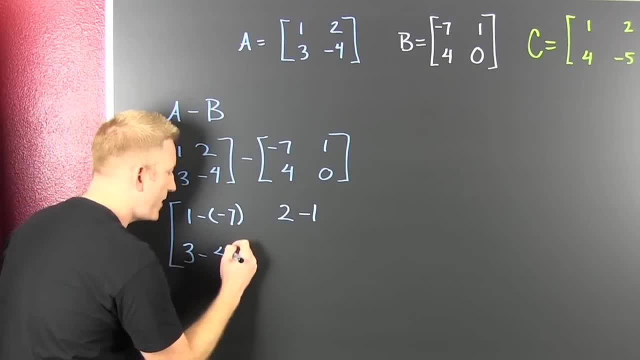 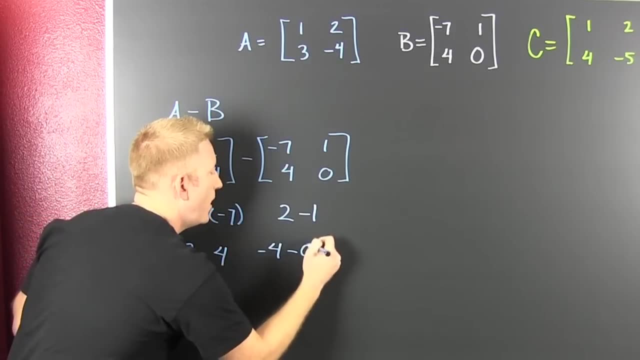 I take my 3. T, T And I subtract off 4. Sure, But wait, There's more. There's that minus 4. Minus, 4. Minus, Oh, finish him, Yeah, finish him. 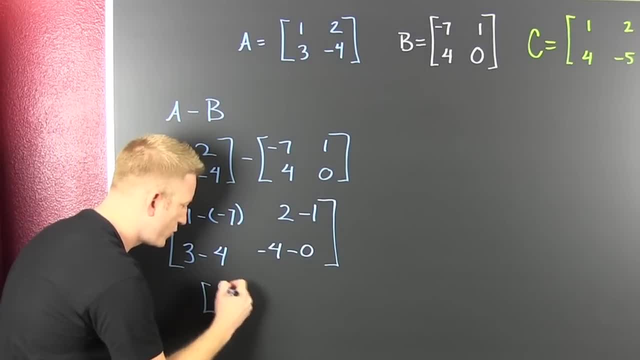 Do the addition 1 minus a minus 7 is 8.. Great, I'm going to have to make that a little bigger. So then 3 minus 4 is a minus 1.. And then 2 minus 1 is 1.. 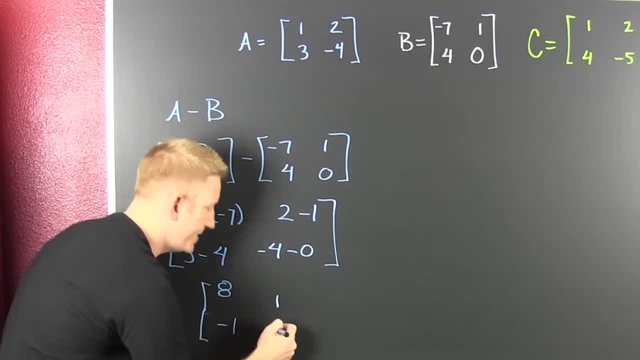 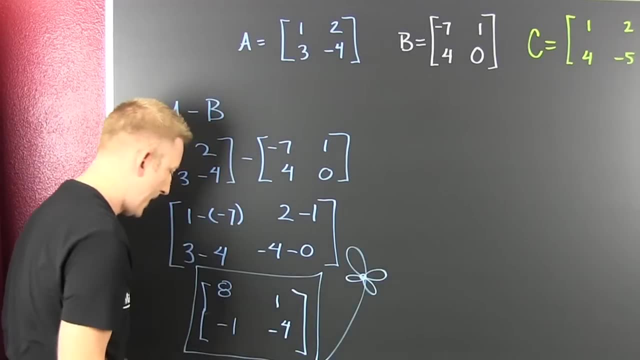 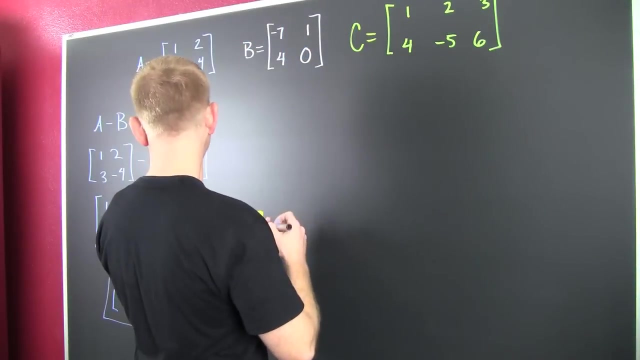 And then minus 4. minus nothing is still a minus 4.. Boxing flower. Nextly, let's go and see some of these additions. It's a new addition. So then, what am I looking for? Let's look for a plus b. 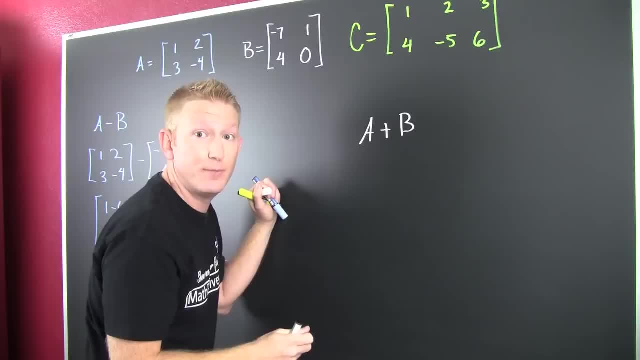 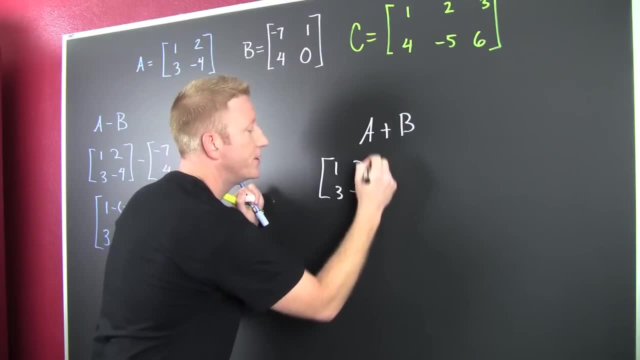 Yeah, that says we're going to take all the components in a and add them to all the components in b Appropriately. This is 1, 2, 3, minus 4.. Sure, And then I'm going to add it to. 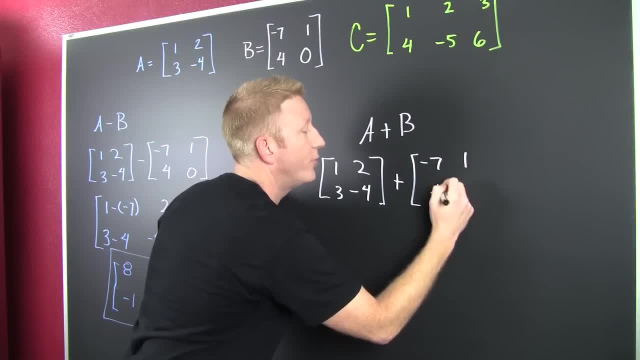 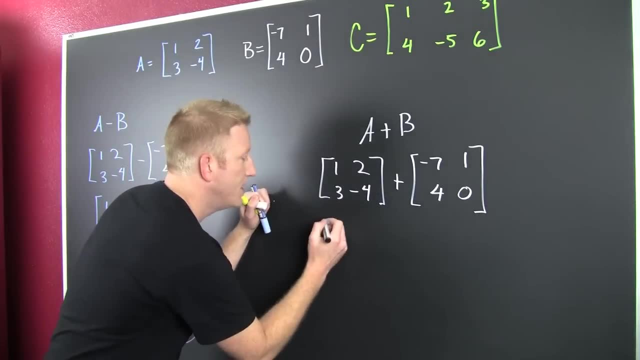 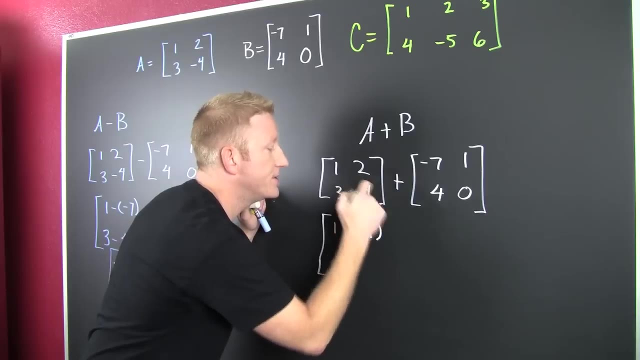 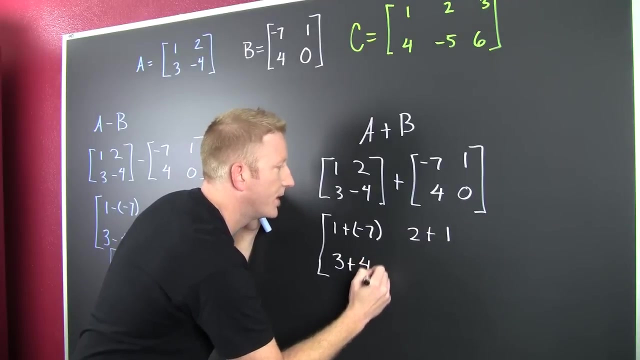 A minus 7,, 1,, 4.. Oh, and we go, and we add them component-wise. So then row 1,, column 1.. This is 1 plus a minus 7,, 2 plus a 1, and then 3 plus a 4, and we go. 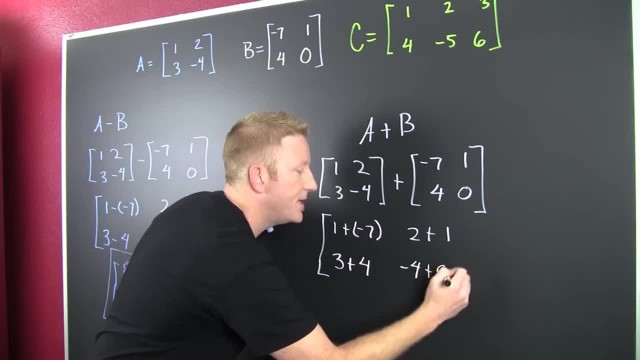 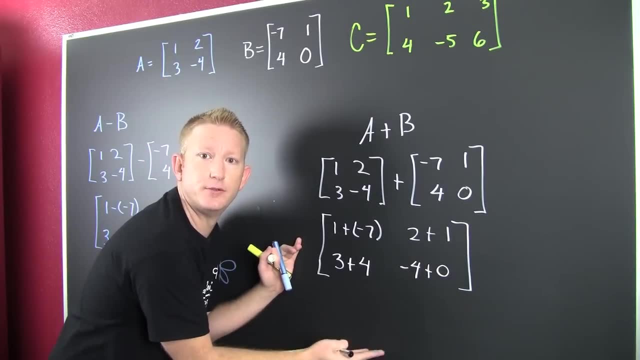 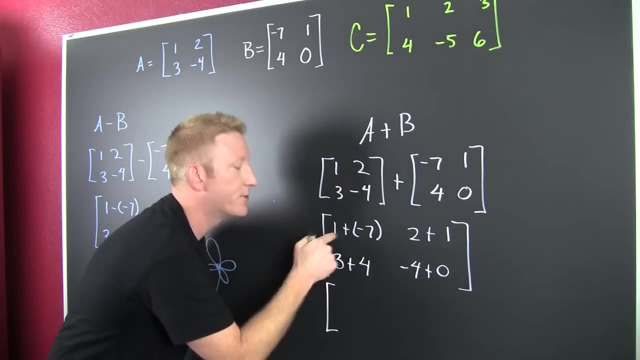 And we take that minus 4, and we add it to a nothing. Finish him, Yeah, finish him, Ooh. is this too low? Oh, over here, No, right here, Okay, So then that's a minus 6.. 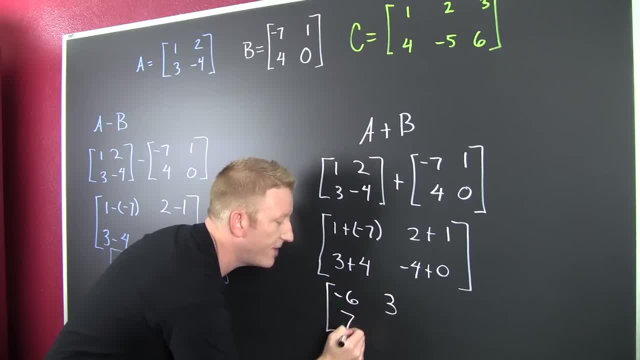 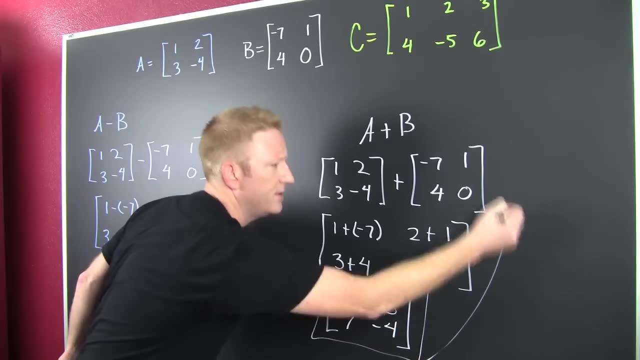 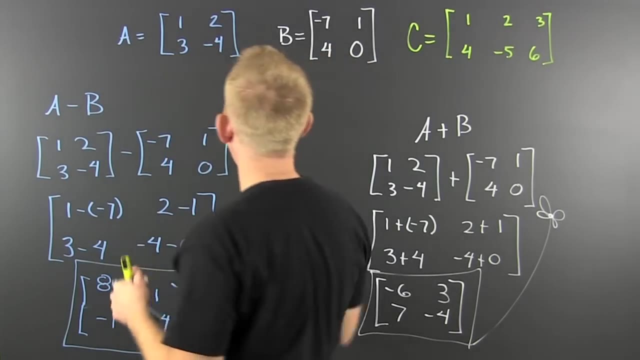 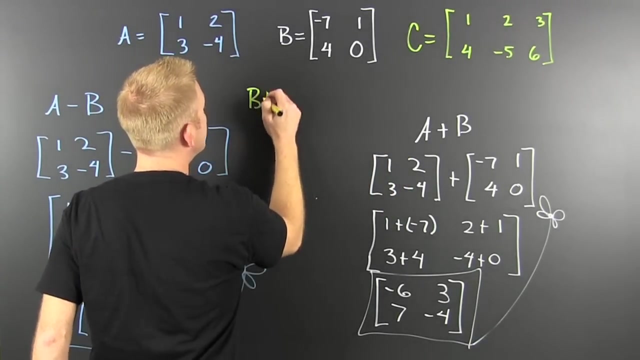 That's a 3. Tee hee, tee hee, 7. And a minus 4. Sure, Sure, One more. Wait a minute. what if I go when I try to add B and C? well, let's see. see B plus C. so 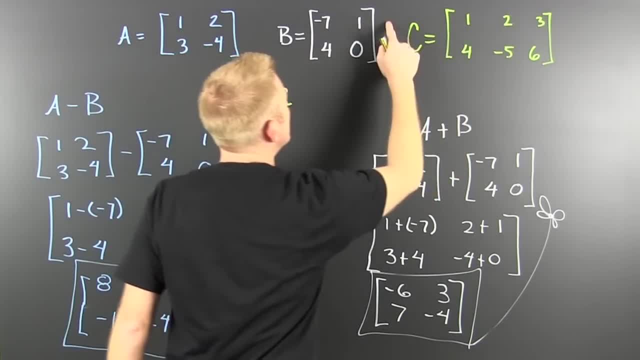 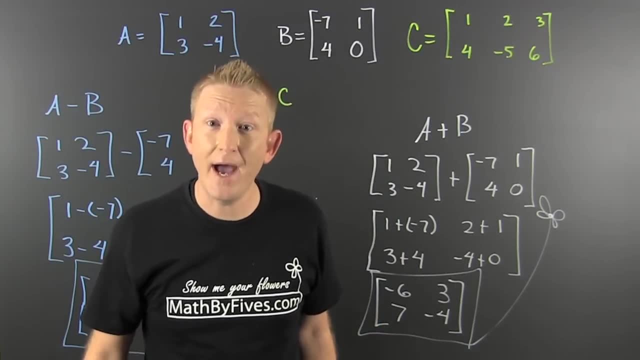 then I take this and I add it to that, I take this and I add it to that and I take: oh, that's whack, you can't add matrices that aren't the same size. it matters.